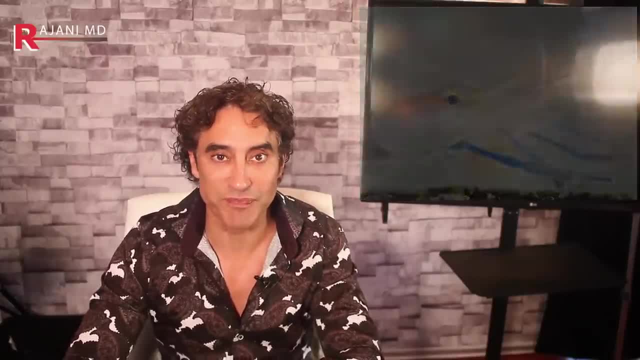 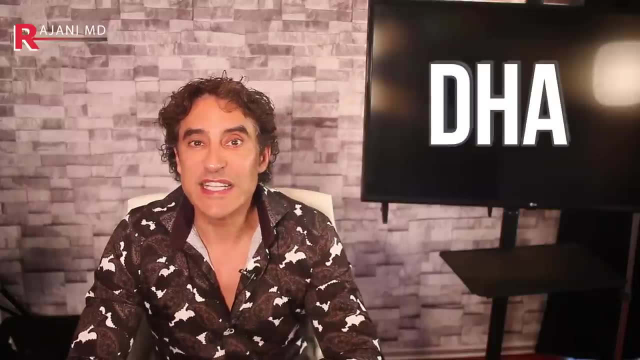 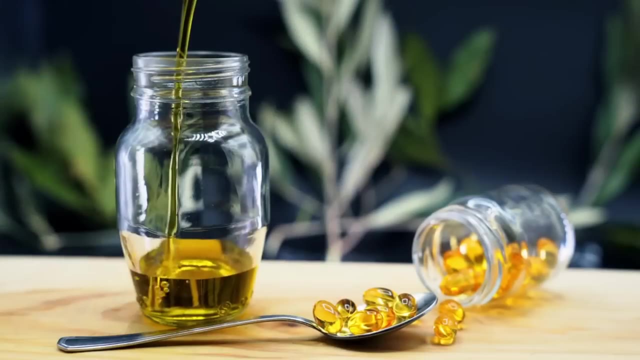 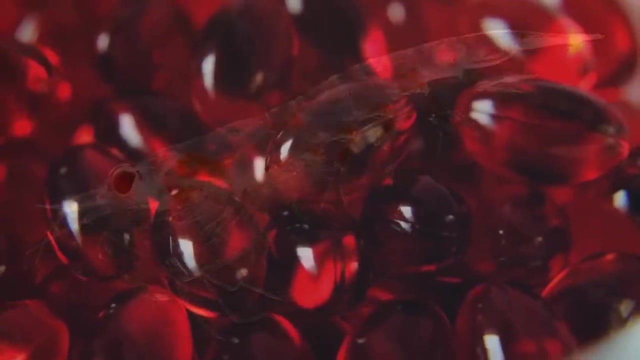 And undergo long Periods of starvation. Number two: they're the best absorbed omega three fats. You see, DHA and EPA from krill seem to be more bioavailable than omega threes from fish oil. This is because the majority of DHA and EPA from krill oil is bound. 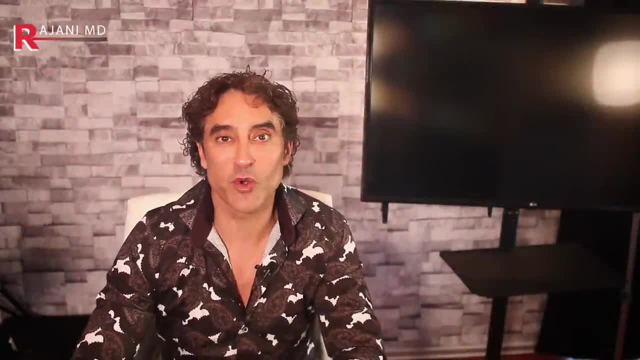 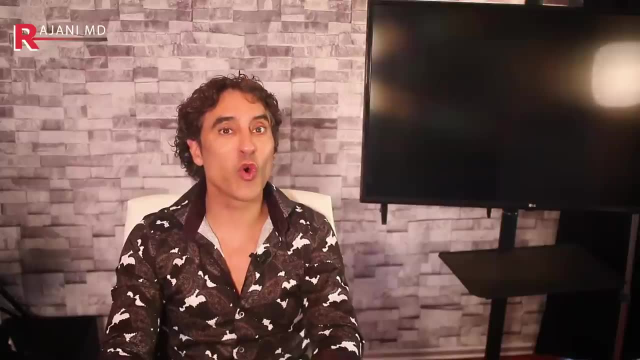 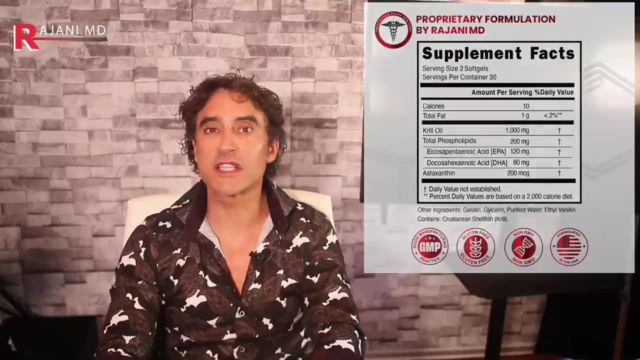 to phospholipids, which are then efficiently absorbed by the body. Number three: Much fish oil that people use is rancid. krill oil is not, And the one I have certainly isn't. You see, oxidation is a normal process in all oils that contain polyunsaturated fatty. 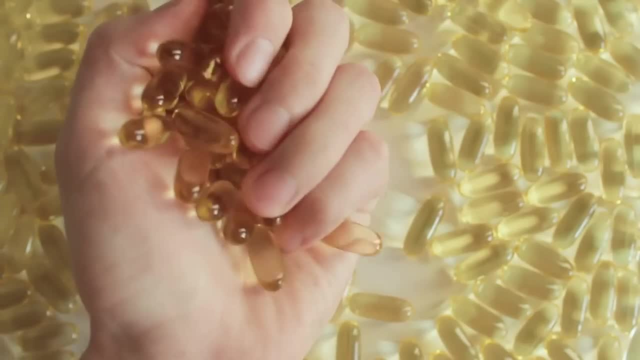 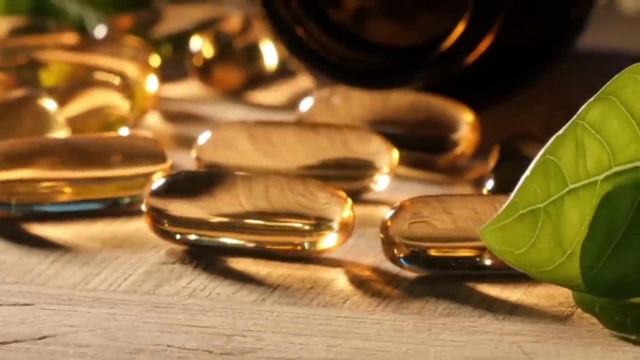 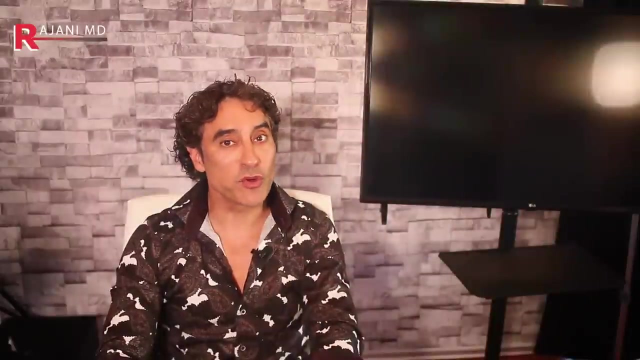 acids. fish. fish oil is particularly susceptible to oxidizing, which happens faster, of course, when it's exposed to heat, air or light- the same three elements We don't want Our skincare being exposed to. it's also prone to oxidization because it's a long 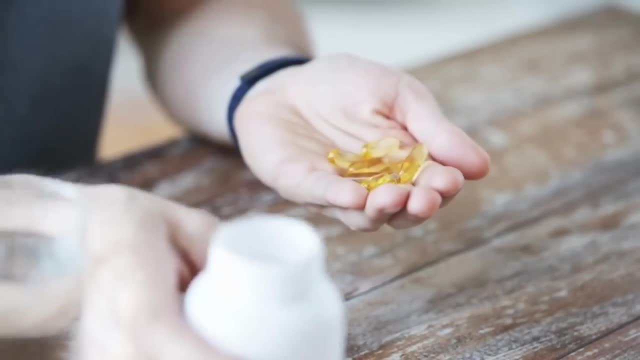 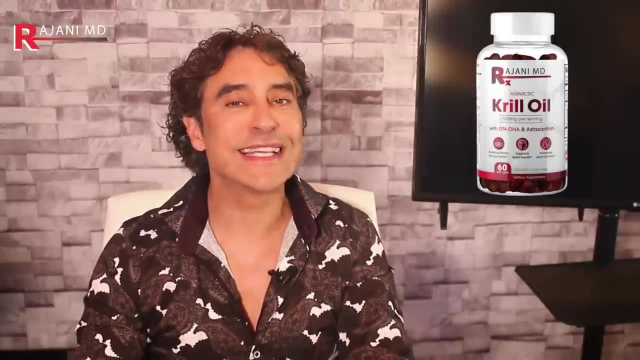 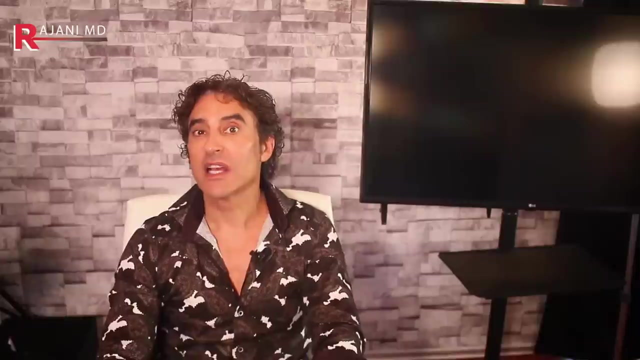 supply chain to get to the end user, and it often lacks the appropriate preventive measures on its way to you. But my number one reason for using krill oil is that it contains astaxanthin. fish oils do not typically contain this element. astaxanthin is one of the most potent and 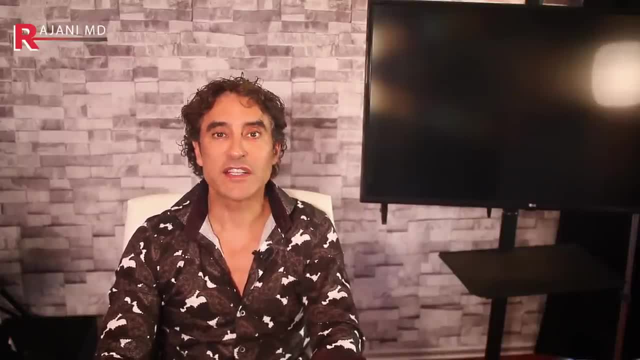 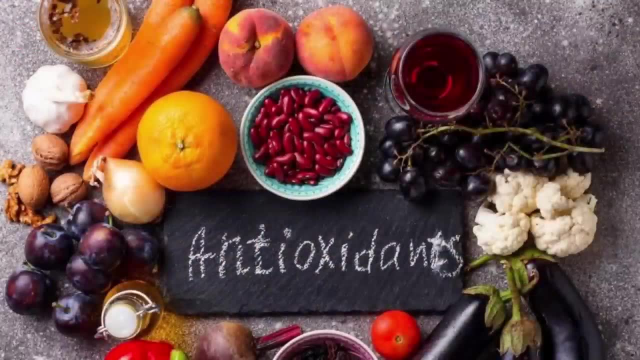 powerful antioxins, Okay, Okay. So the next thing I want to talk about is the anti-inflammatory elements of astaxanthin. The anti-inflammatory elements of astaxanthin are based on its antioxidant properties, among others, and it has been proven to benefit. 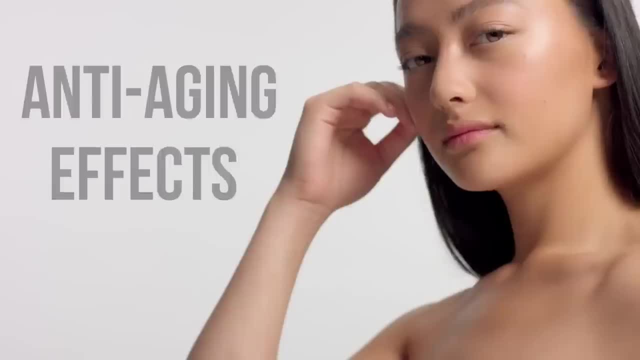 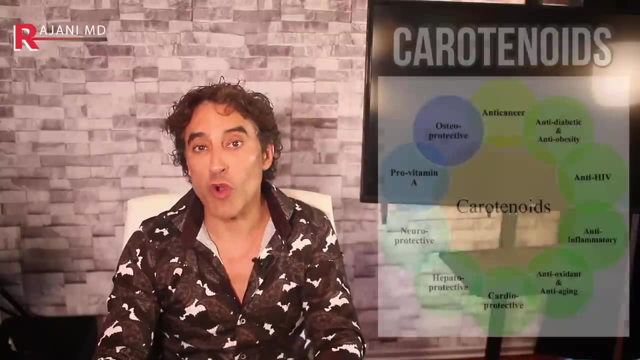 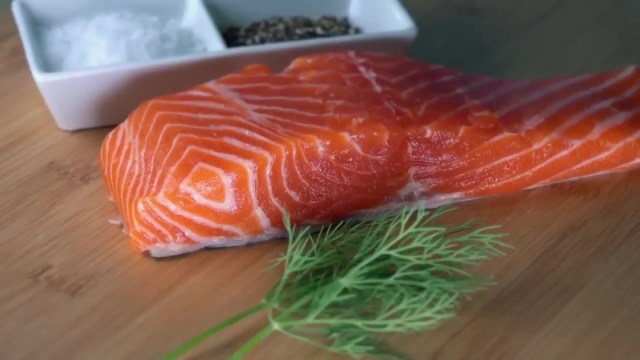 And improving health, and it's used often for its anti-aging effects. Astaxanthin is the red pigment that belongs to the group of chemicals called carotenoids. It occurs in certain algae and causes that pink or red color that you see sometimes in salmon, but it's a 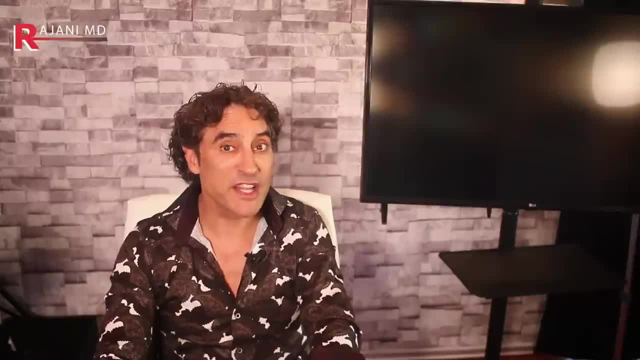 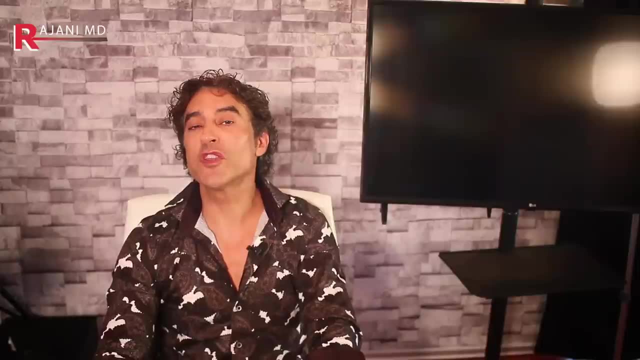 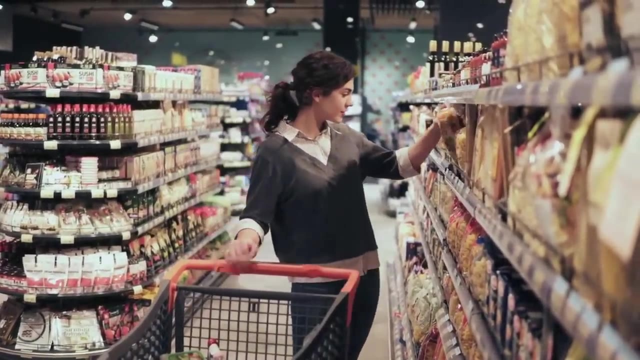 Abundant in krill. If you watch my video on farm salmon and the difficulty finding real wild caught salmon, you know that often there's fake coloring to mimic this in many of the foods we see on the shelves that are grocery store and beyond. We do not want fake, We do not want synthetic, We want the real deal. And it just happens to be found in krill and is the most bio available. Okay, The benefits of astaxanthin include immune system support. Astaxanthin can influence your immune system, helping to activate white blood cells, T cells and natural killer NK cells. reduction in inflammation, along with boosting in the immune system. 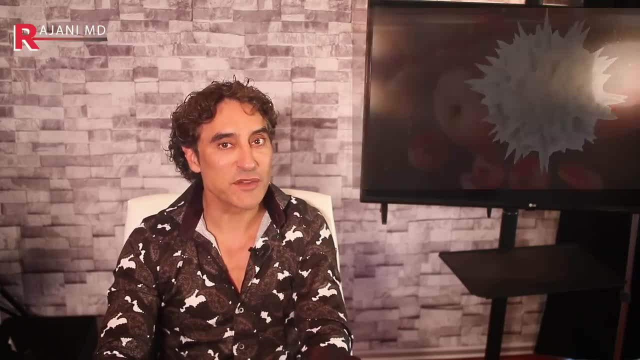 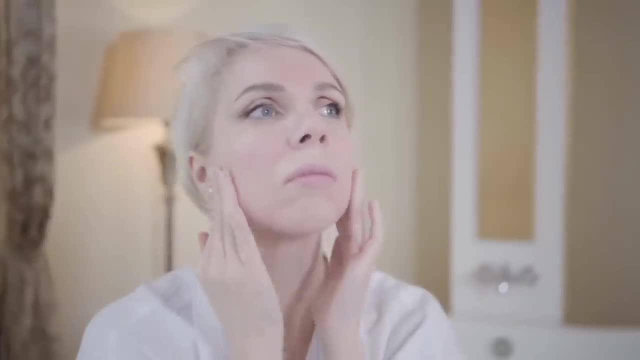 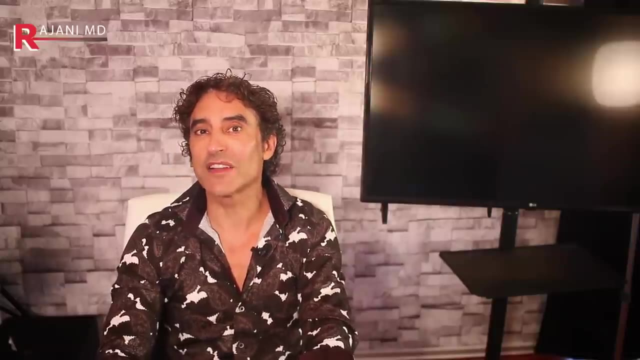 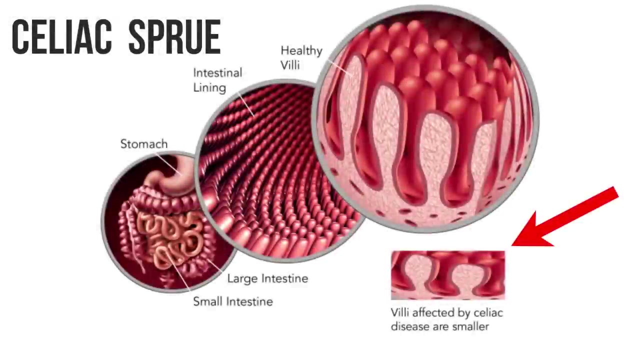 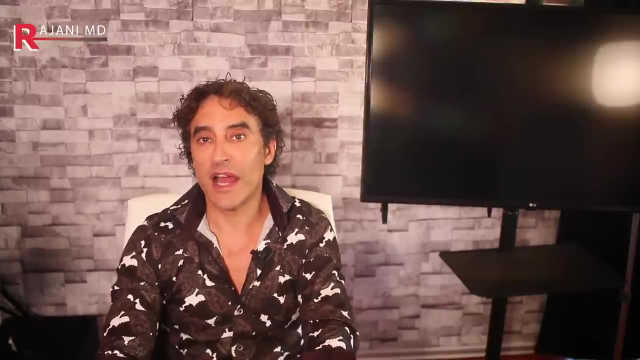 Astaxanthin may also help reduce inflammation. We know inflammation leads to aging. It's part and parcel of what causes heart attack, stroke and, of course, aging in the skin, Which we're concerned with on this channel in particular, this pigment acts on the reactive oxygen species to reduce proteins that can cause inflammatory diseases like celiac, sprue, rheumatoid arthritis, heart disease and diabetes- all very common uh ailments affecting so many people. 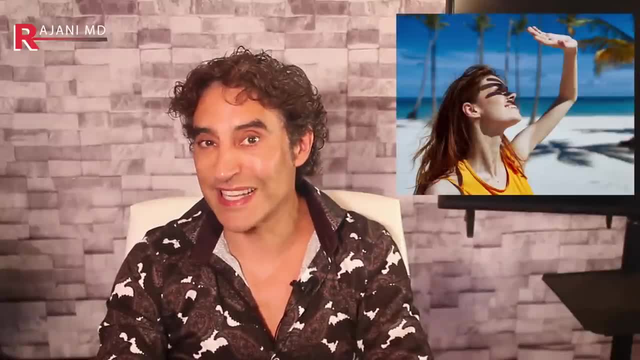 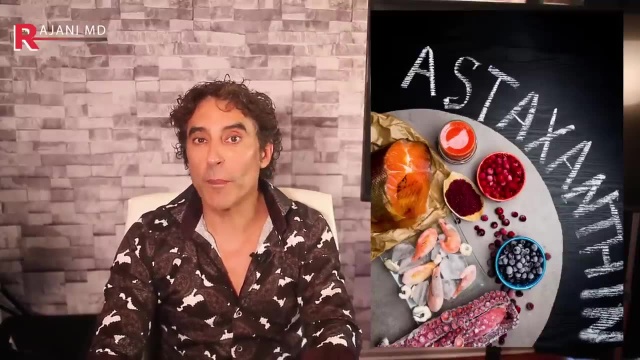 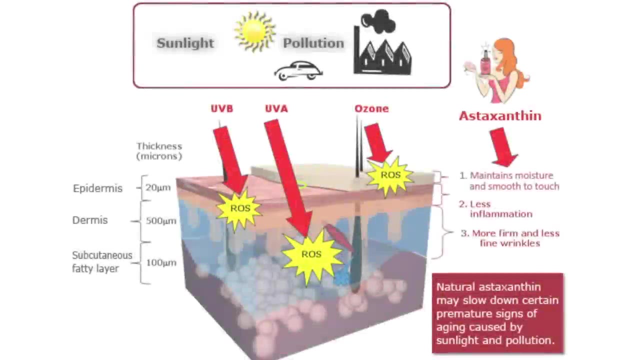 There's also evidence that there's protection from UV skin damage by taking supplements or consuming foods Rich Astaxanthin may also help protect your skin from UV damage, Number one cause for skin aging. Of course, as we know, astaxanthin accumulates in the epidermis and dermis layers of your skin, helping to block UV penetration and reduce existing sun damage. support cognitive health. 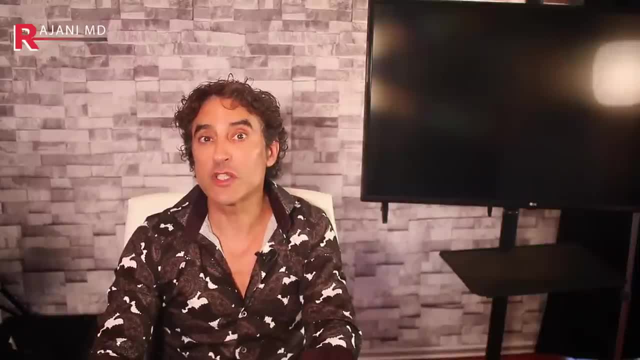 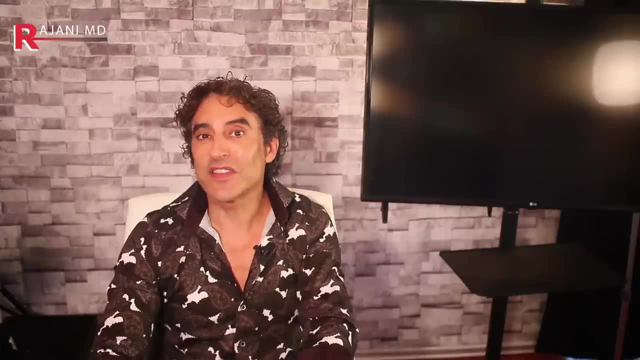 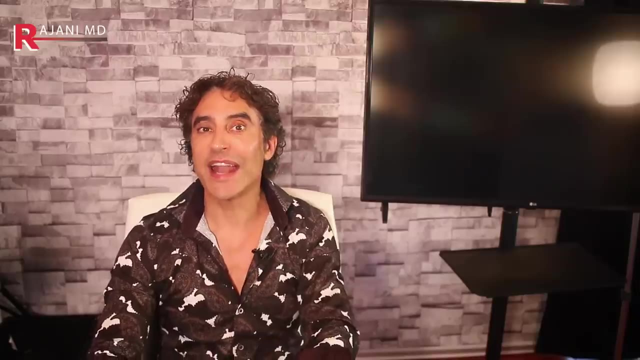 Another great reason for astaxanthin: carotenoids have positive effect on the brain by reducing risk for neurodegenerative Okay Diseases. Astaxanthin is a smaller molecule, which means it actually can cross the blood brain barrier and that adds protection for your brain as well as your body's organs. 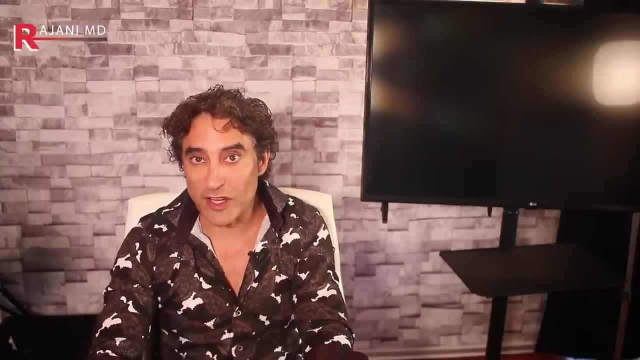 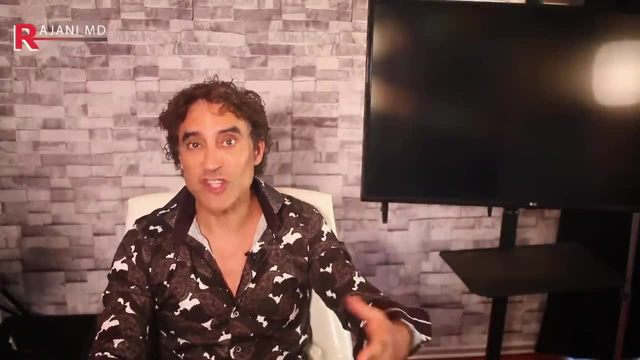 You see, not everything can cross that barrier. It's a well-known barrier and many supplements and elements are purported to be helpful for cognition and mentation, but they actually can't cross the blood brain barrier like this. This carotenoid may also help. 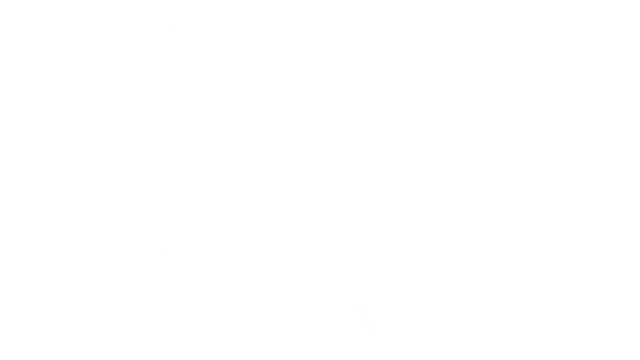 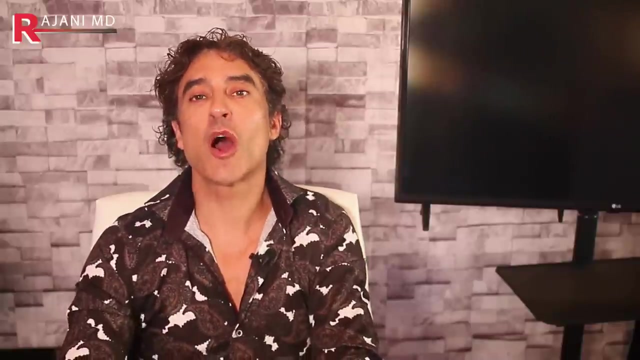 Okay, Alzheimer's disease and other cognitive disorders and slow or kind of abate their onset. Healthy heart function is a common one You hear of. if you're trying to improve your heart health, you may have good results with astaxanthin. 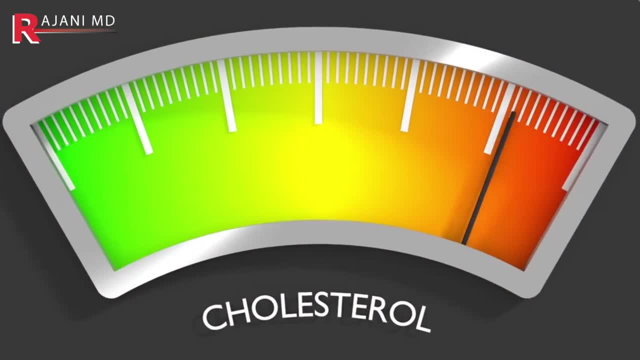 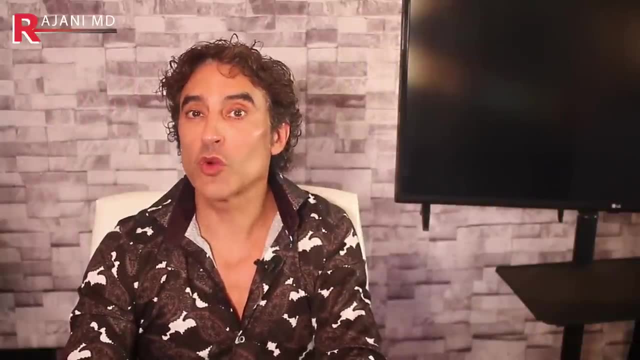 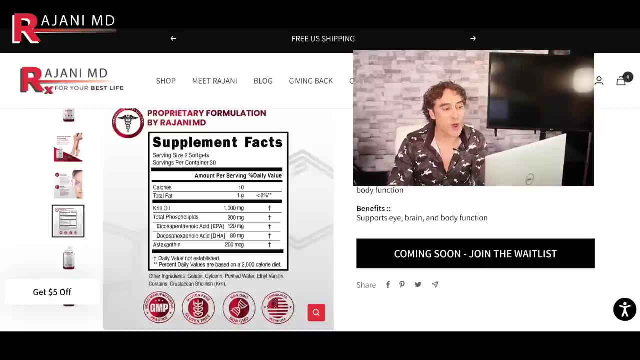 This carotenoid can help reduce LDL, or that bad cholesterol, and can raise the HDL, or the good cholesterol, while also lowering blood pressure. So how much do I take? Let's look on the label of mine. So if you look, here, there's 1000 milligrams of krill oil.